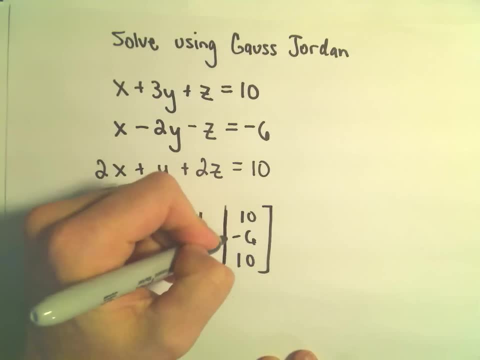 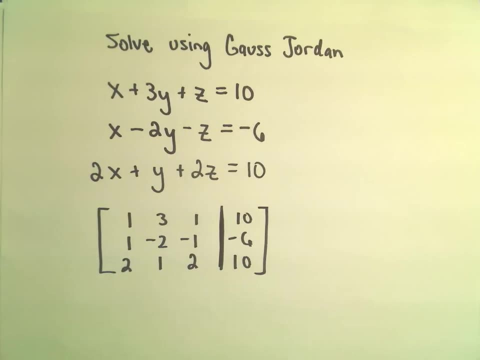 So, again, our goal is to make the left side of this matrix look like the identity matrix: 1, 0, 0, 0, 1, 0, 0, 0, 1.. So we're going to have to do a few things to do that. 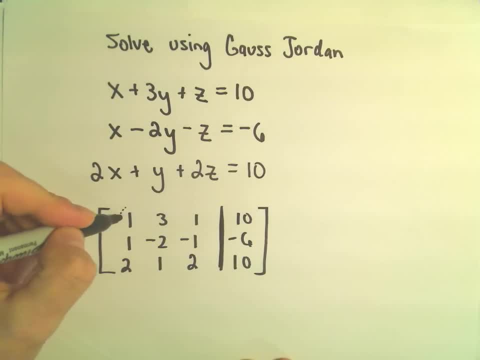 Well, the first thing I want is typically, I want to get a 1 in the top left corner, which okay, great, we have that. But my next entry is: I want to get zeros in the rest of the column. So I'm going to do two steps here at once. 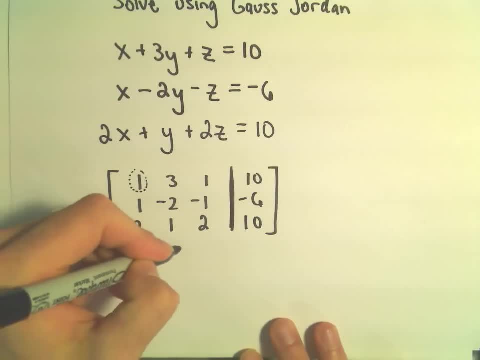 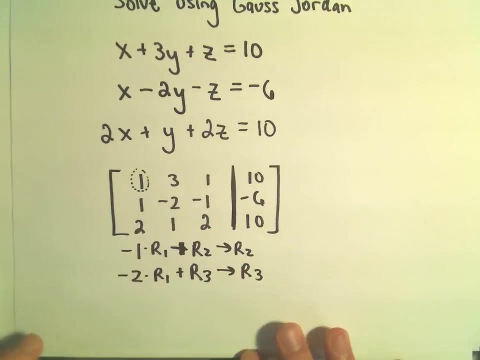 So I'm going to take negative 1 times row 1, add that to row 2, and that's going to give me my new row 2.. I'm also going to take negative 2 times row 1 and add that to row 3 to get my new row 3.. 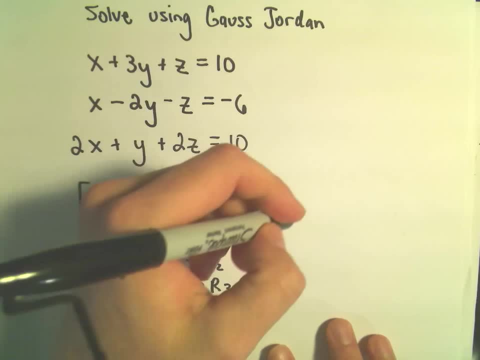 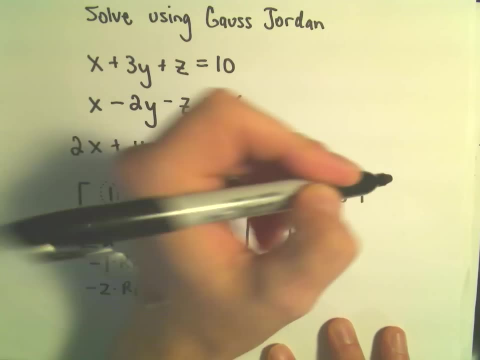 Okay, so if we do this, let's maybe move off to the side here. If we do this, Okay, So we're not going to do anything at all. to the first row. So we have 1,, 3,, 1, and 10.. 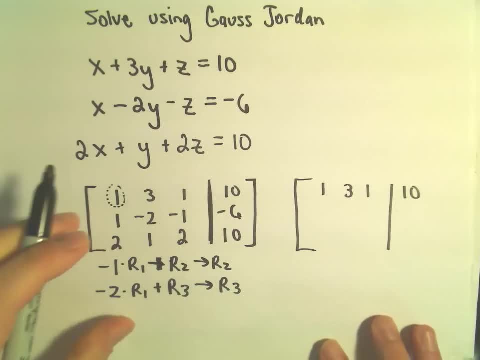 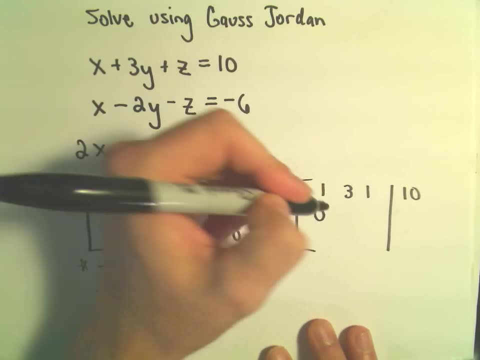 So that doesn't change. But then I'm going to take, I'm going to do my first step here. So if we take negative 1 times 1, we'll get negative 1 plus 1, which is 0.. That's what we wanted. 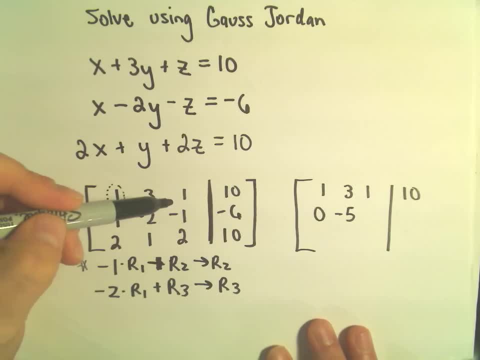 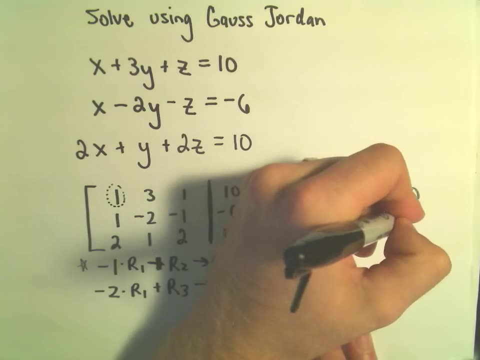 We'll get negative 3 plus negative 2, which is negative 5.. We'll get negative 1 plus negative 1, which will be negative 2.. And then we'll get negative 10 plus negative 6, which will be negative 16.. 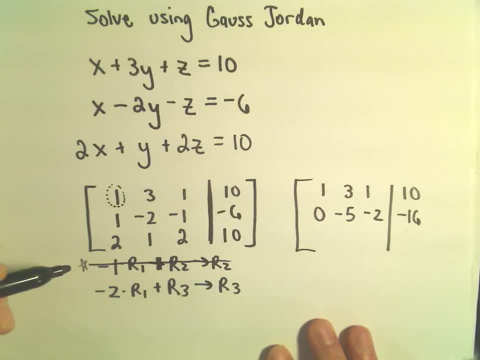 So that takes care of that operation, that step. If we do negative 2 plus 2, we'll get 0.. Negative 2 times 3 is negative 6. Negative 6 plus 1 will be negative 5. Negative 2 times 1 will be negative. 2 plus 2 will be 0.. 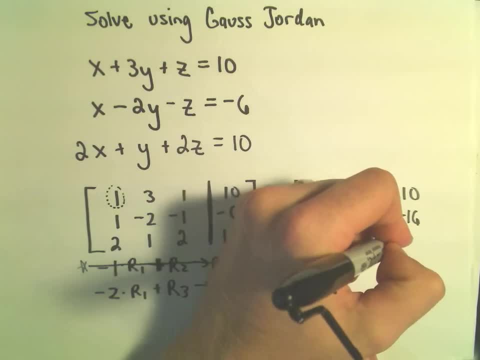 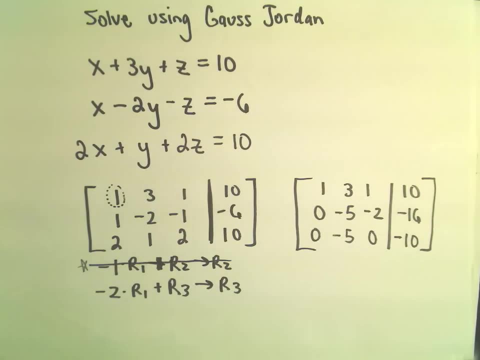 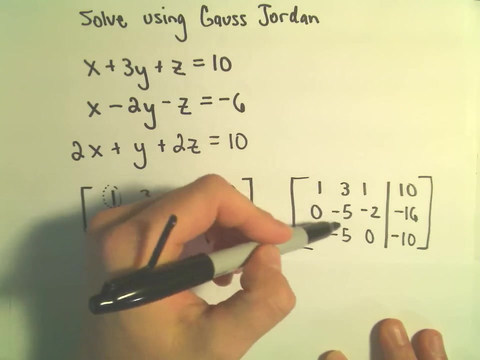 And then we'll get negative 20 plus 10, which will be negative 10.. All right, So a couple different things we could do here. Again, I want to eventually make a 1 appear sort of in the middle here, But what I'm going to do, I think I'm going to interchange row 2 and row 3.. 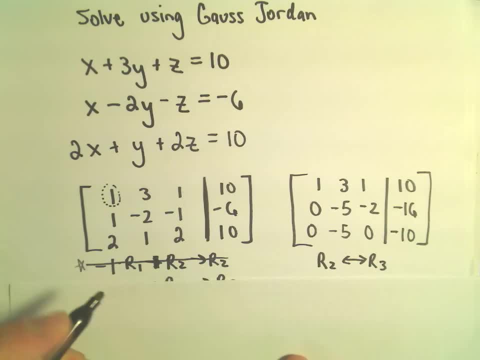 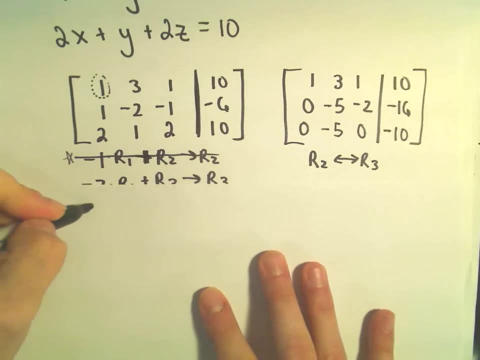 I'm just going to switch those out. So if we interchange row 2 and row 3, well, again nothing happens to our first row. So we still have 1, 3,, 1, 10.. But now I'm just going to interchange. 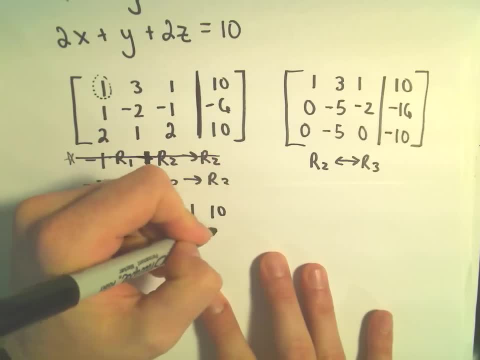 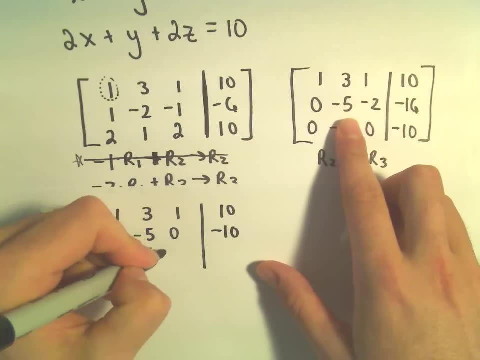 So I'll have 0,, negative 5,, 0, and negative 10.. That will be my second row, And then we'll have 0,, negative 5,, negative 2, and negative 16 as our new third row. 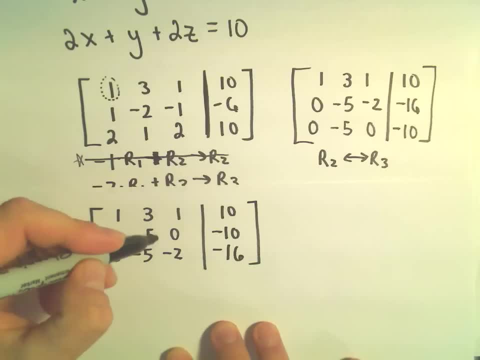 So we just switched them out. Well, to make a 1 appear in our second place, eventually I'm going to divide both sides by negative. Excuse me, I'm going to divide row 2 by negative 5. But eventually I want to get a 0 above it and below it. 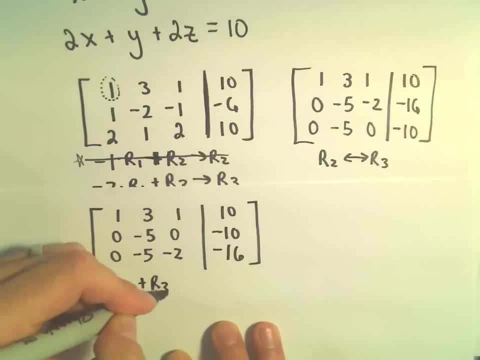 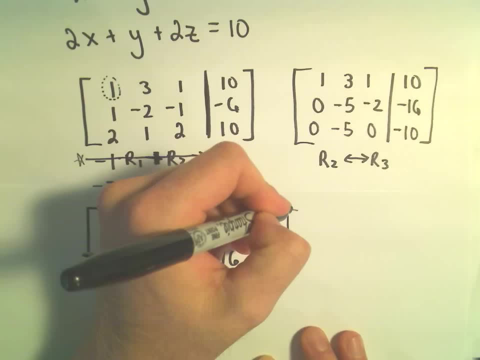 To make that happen, I'm going to go ahead and add row 2 and row 3 to get my new row 3.. So this is kind of the thing with matrices: There's sort of lots of different ways that you can go about doing it to eventually get all to the same answer. 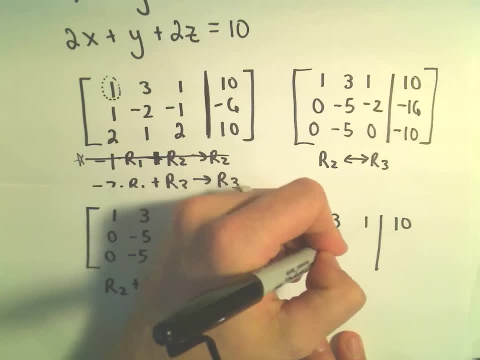 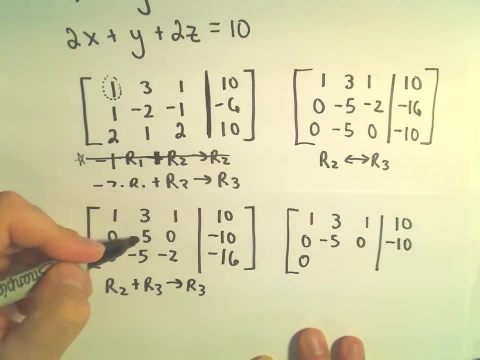 So I'm leaving the first row alone. I'm leaving the second row also alone for the moment, But if I add row 2 and row 3, I'll get a 0.. Negative 5 plus negative 5 is going to be. 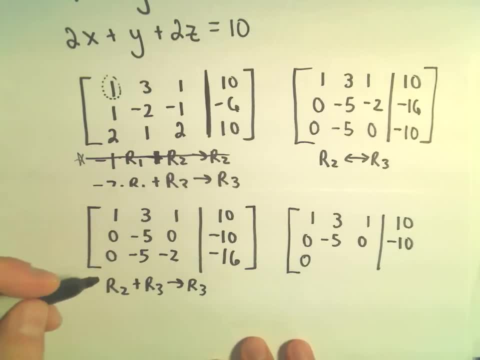 Okay, well, let's be careful, right, Because we don't want to just add them. So I think what we're actually What we need to do is I'm going to take row 2 and multiply it by a negative 1.. 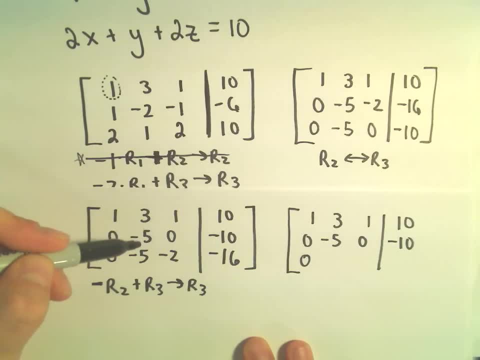 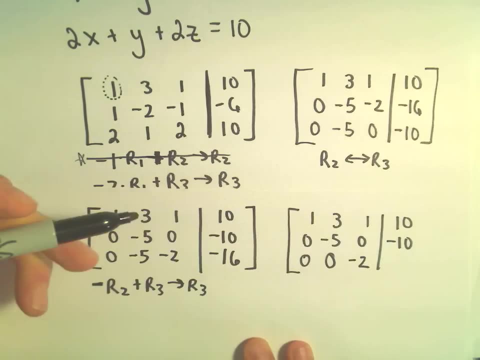 That's going to do it for us, Because then I'll get a positive 5 plus negative 5, which will give us a 0. And then we'll get 0 plus negative 2, which is well negative 2.. 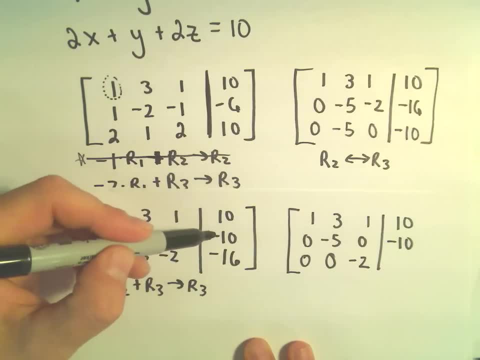 And if we take negative 1 times negative 10, we'll get positive 10.. 10 plus negative 16 will give us a negative 6.. All right, so let's see. The next thing I am going to do is I'm going to make this negative 5 into a positive 1.. 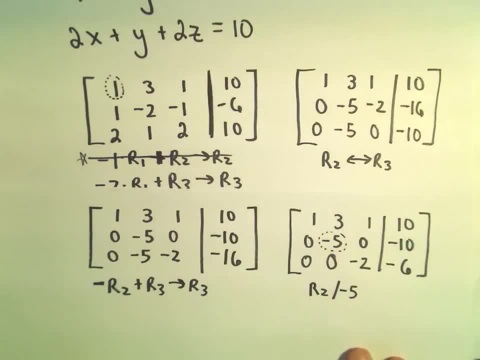 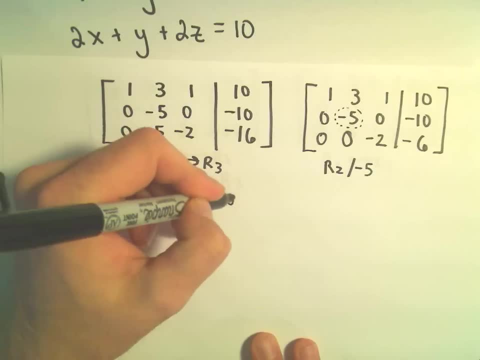 And I'm going to do that by taking row 2 and dividing that by negative 5.. So if we do that again, the first row we're just leaving it alone. The second row will now become 0, 1, 0.. 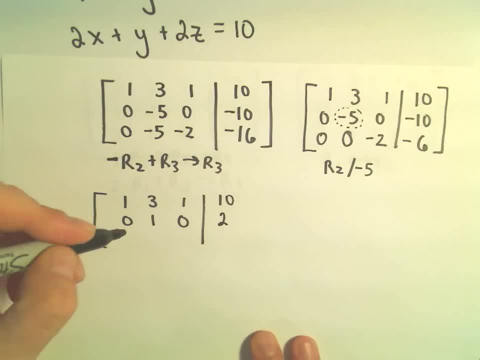 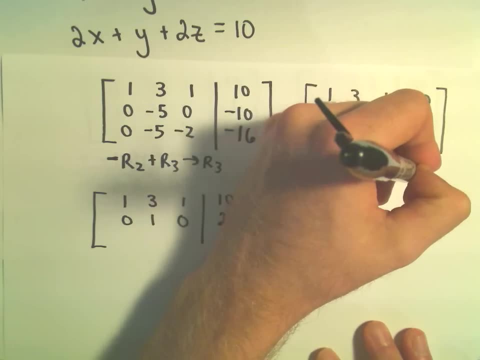 And we'll get a positive 2.. And let's see, I'm going to go ahead and even I think I'm going to do another step at once as well. I'm going to take row 3 and divide that by negative 2.. 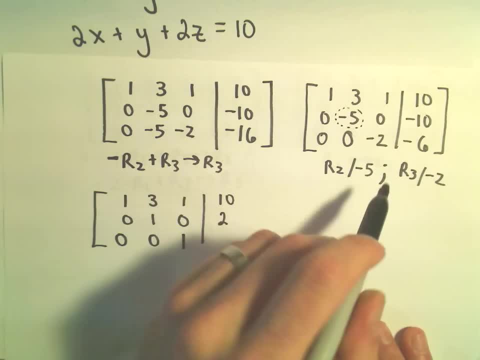 So we'll get 0,, 0,, 1.. And then it looks like negative 6 over negative 2 would give us positive 3.. So we're getting pretty close here. In fact, we now know what z should equal. 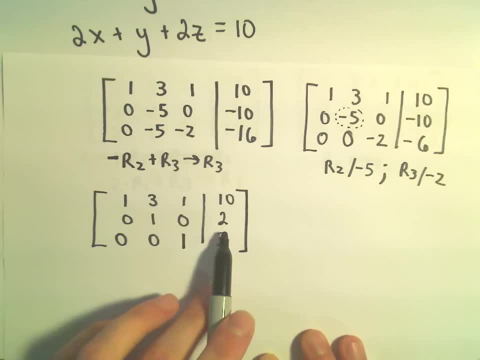 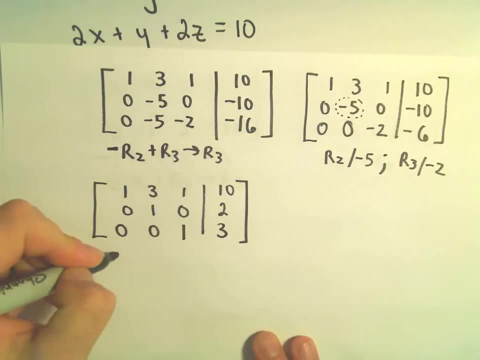 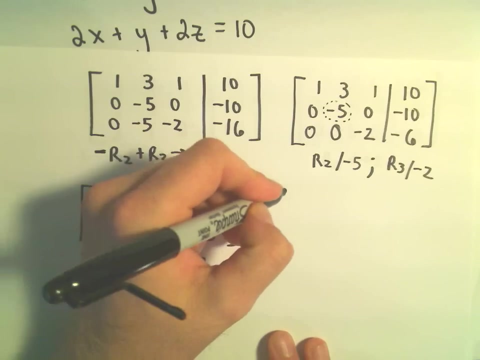 It says z should equal 3.. 1y would equal 2.. But let's go ahead and figure it out. Let's make the left side look like the identity. So I'm going to take negative 3 times row 2 and add that to row 1 to get my new row 1.. 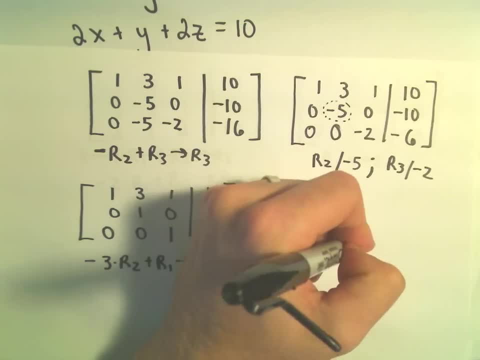 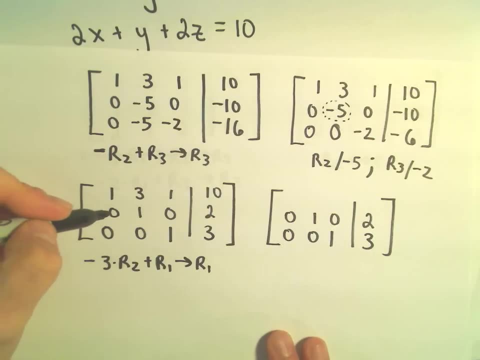 So let's see The second row: 0, 1, 0, 2,. I'm going to leave that alone. The third row, I'm going to leave alone for the moment as well. Let's see So: negative 3 times: 0 is 0 plus 1 is 1.. 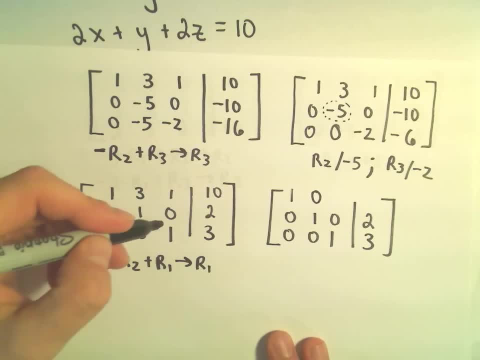 Negative 3 times 1 is negative. 3 plus 3 will give us 0.. Negative 3 times 0 plus 1 is 1.. And then we'll have negative 3 times 2, which is negative 6. Negative 6 plus 10 will give us a positive 4.. 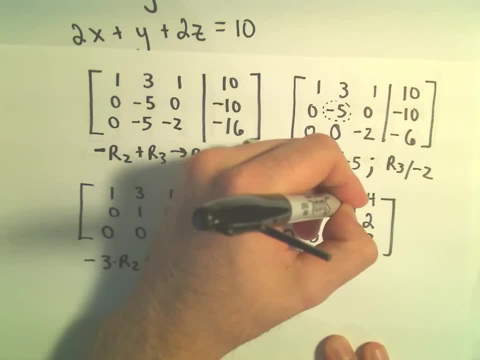 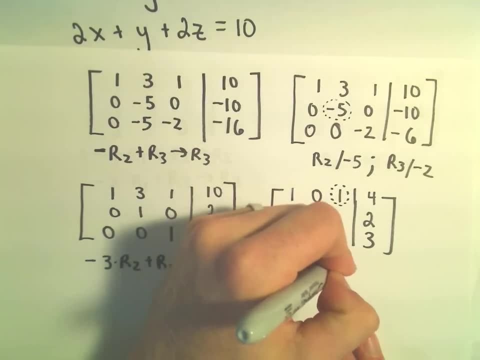 One more step to do. We want to make a 0 in this entry. Well, again, I can just take negative 1 times row 3, add that to row 1, and that will give me my new row 1.. 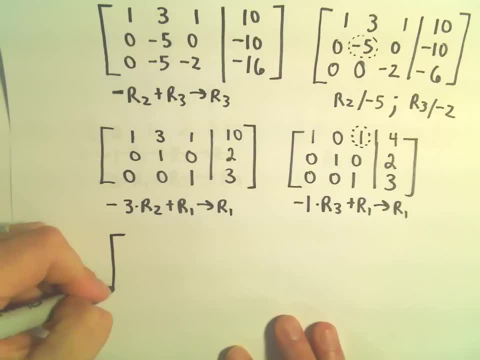 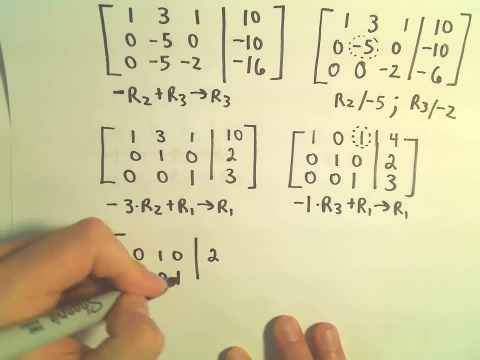 And at that point I think we'll be in business. So the second row: 0, 1,, 0, 2, we'll leave that alone. The third row: 0, 0, 1, 3, we're going to leave that alone. 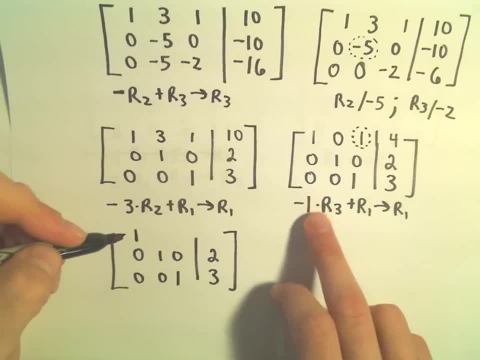 If I take negative 1 times 0 plus 1, we'll get 1.. We'll get a 0.. If we take negative 1 times 1, we get negative 1 plus 1.. We'll get 0..